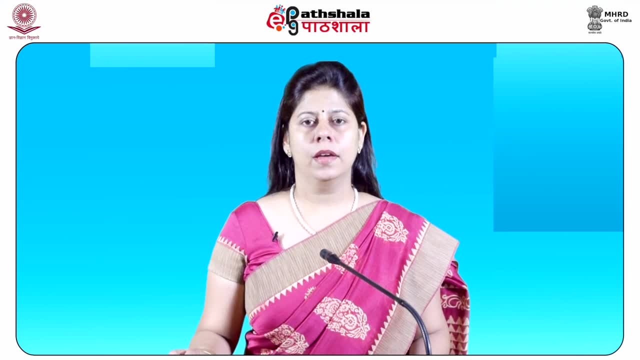 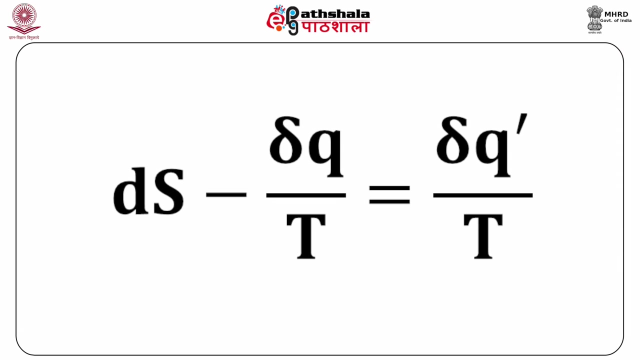 described by equation of heat, The equation of inequality as ds is greater than del Q by T, which is based on the direction of spontaneous process. Clausius suggested different form of second law of thermodynamics based on equality, That is, ds- del Q by T is equals to del Q' by T. 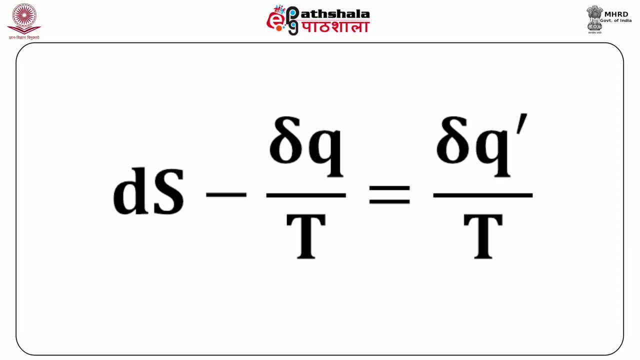 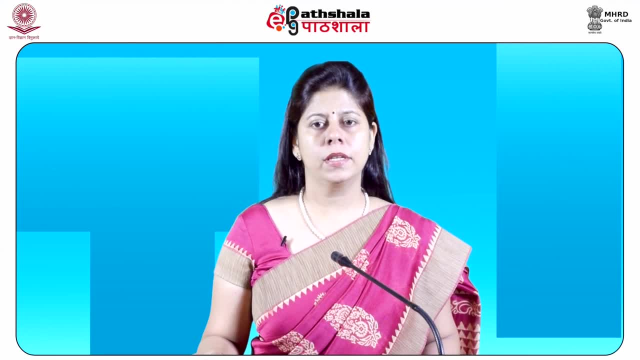 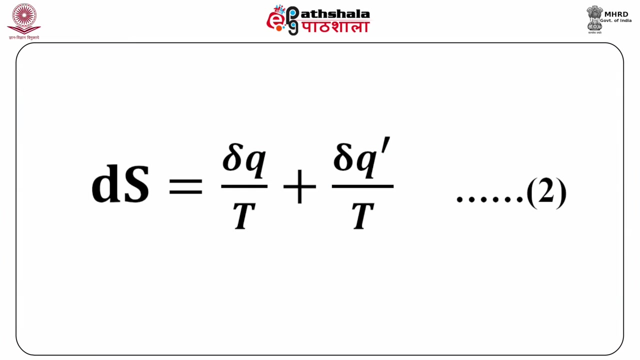 Where del Q' is uncompensated heat, It is not the actual heat absorbed or evolved by the system, but the heat that could have been absorbed in a reversible process in addition to non-equilibrium quantity del Q. in order to maintain equality, Rewriting the above equation ds is equals to del Q by T plus del Q' by T for reversible. 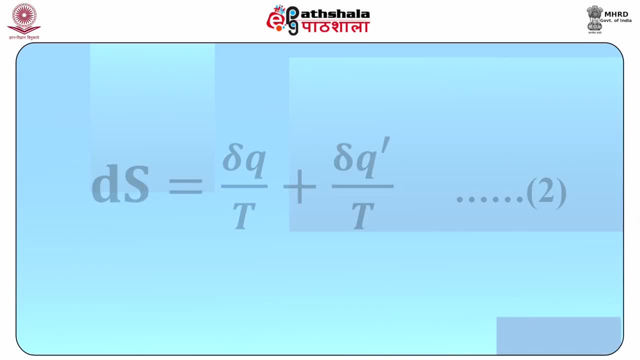 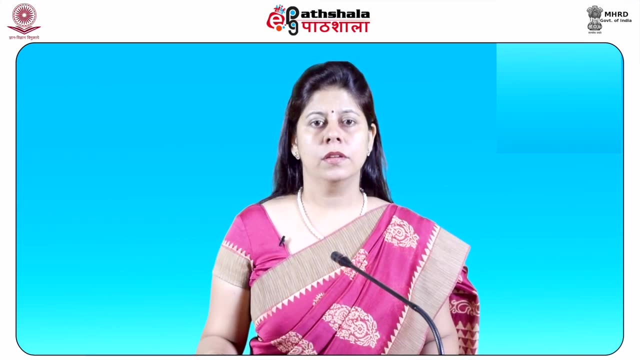 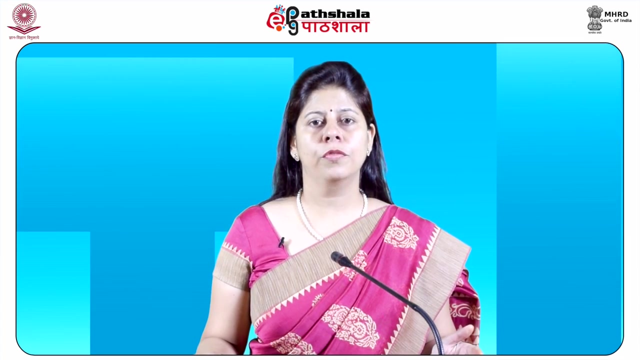 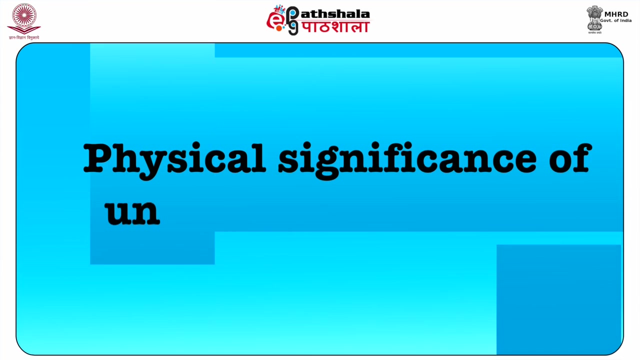 process del Q' is equals to 0, while for irreversible process del Q' is greater than 0. Thus, del Q' is always positive and is produced in the system as a result of non-equilibrium process resulting in an irreversible change. Now we will see the physical significance of uncompensated heat. 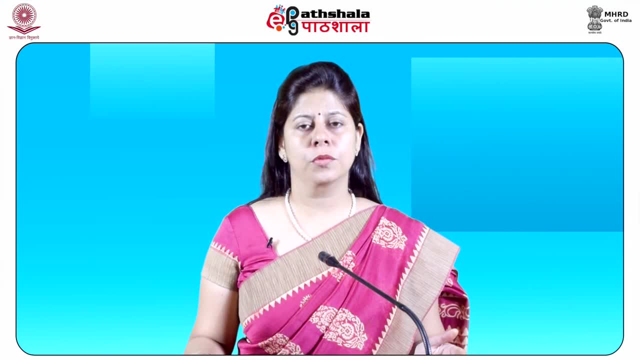 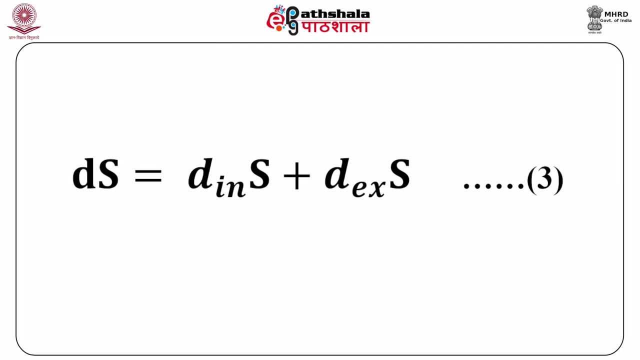 The total entropy change of the system is the sum of two components, ie ds external, which is due to the absorption of heat reversibly from outside, and ds internal, which is due to the irreversible change occurring in the interior of the system. This means ds-total is equals to ds-internal plus ds-external. 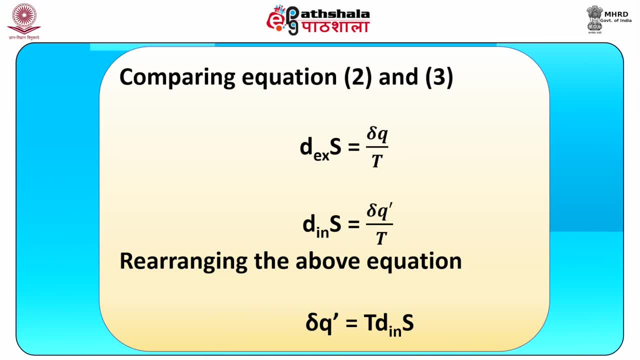 compare-equivalent equation 2 and 3, we have: ds external is equals to del Q by T and ds internal is equals to del Q prime by T. Rearranging the above equation gives: del Q prime is equals to T ds internal. 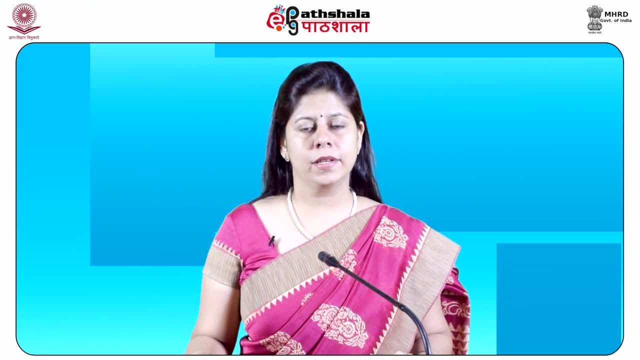 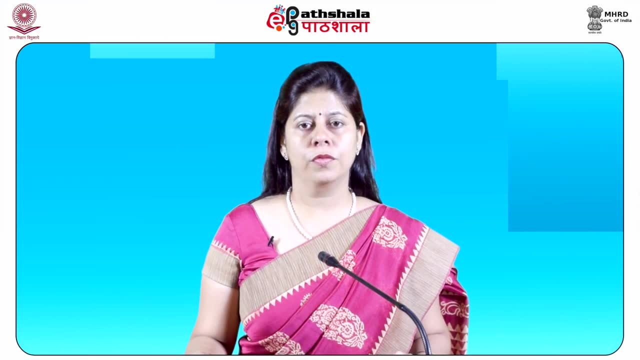 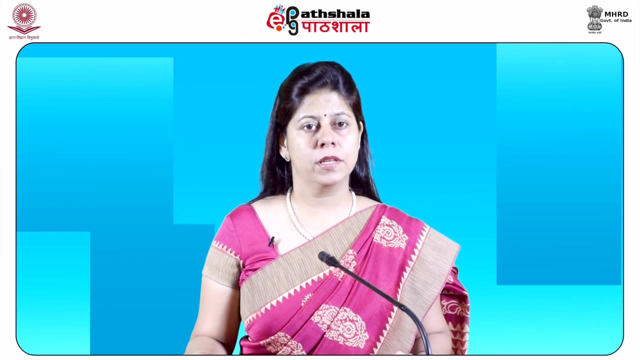 Thus, from this equation, we can say that the uncompensated heat is related to the production of entropy as a result of some irreversible processes occurring within the system. Such processes can be mixing of gases, diffusion of solute from higher to lower concentration. 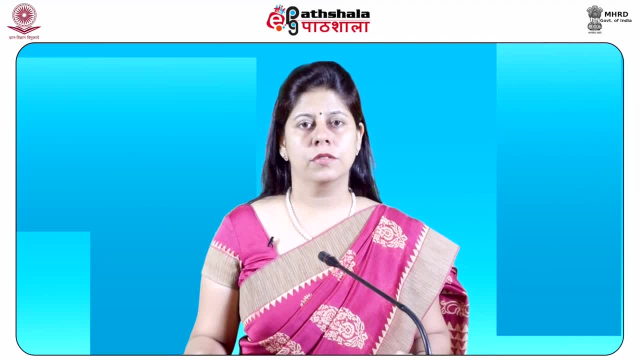 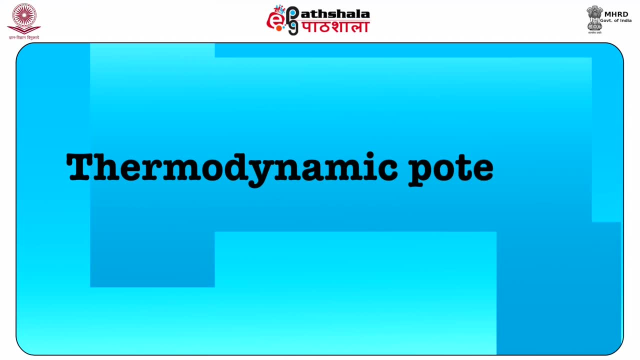 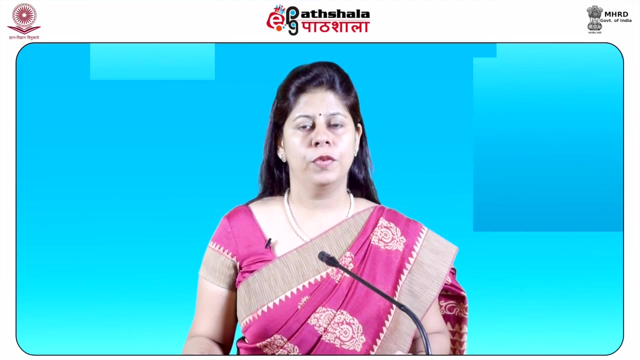 The randomness in the system increases as a result of increase in the disorder in the state of system. Thermodynamic potential At equilibrium Responsive parameters u, s, v and ni are function of state, and linear combination of these parameters are also state functions. 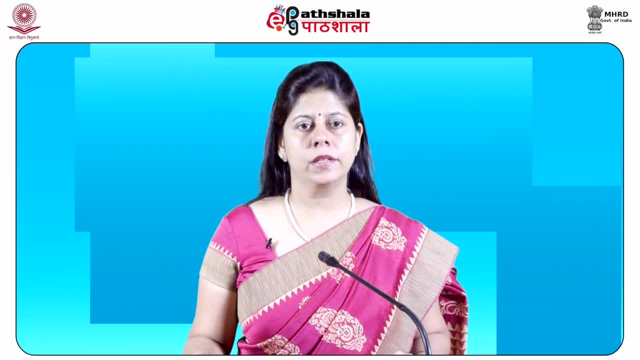 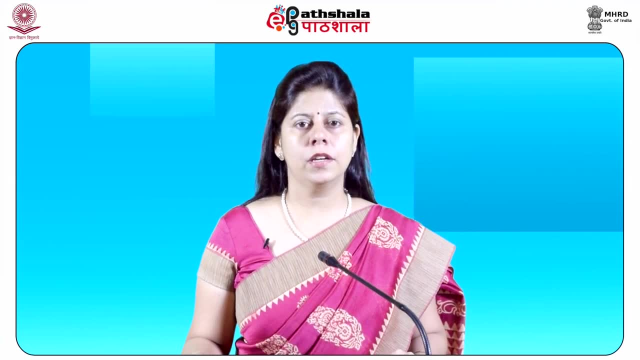 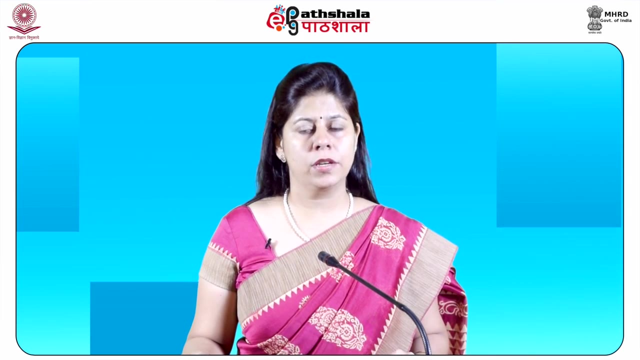 Helmholtz, Gibbs and others have considered such combinations and have found that these are often more useful than the internal energy for describing systems under ordinary experimental conditions. Such combinations are called thermodynamic potentials. They are extensive quantities and must not be confused with the ordinary potentials, which are derivatives of thermodynamic. 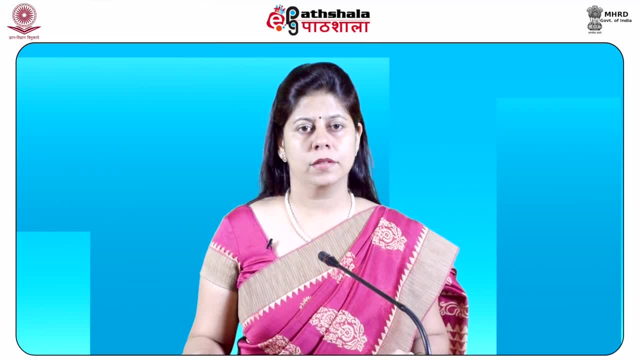 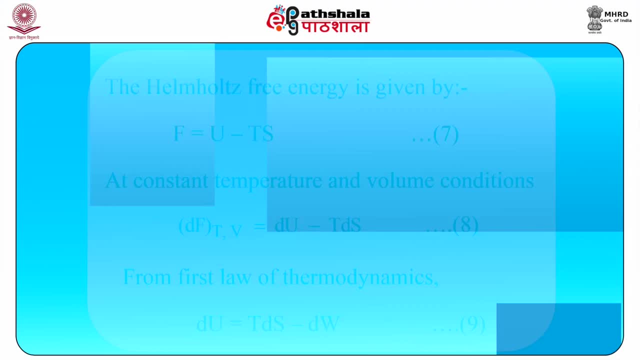 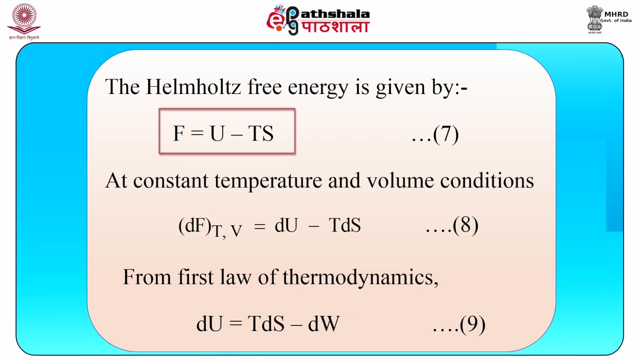 potentials and are intensive quantities. Some of these thermodynamic potentials are Helmholtz free energy. The Helmholtz free energy is given by the expression. F is equal to U minus Ts At constant temperature and volume conditions. we can write the differential: 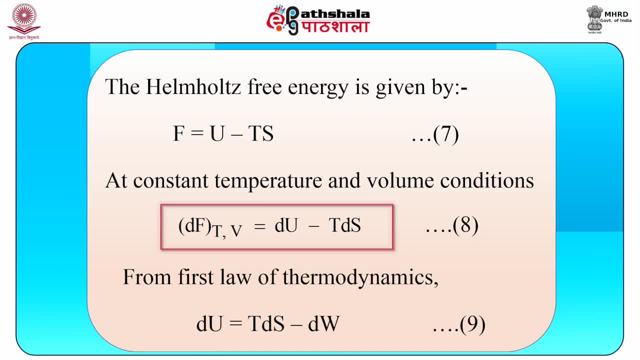 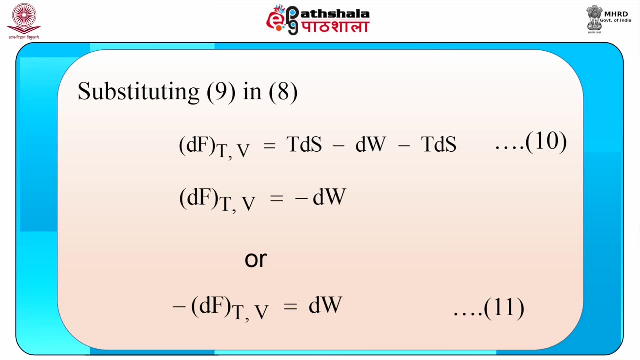 form, as dF is equal to du minus Tds. From the first law of thermodynamics, du is equal to Tds minus dw. Substituting this equation in the previous one, we get dF is equal to Tds minus dw minus Tds, and therefore we get dF is equal to minus dw at constant temperature. 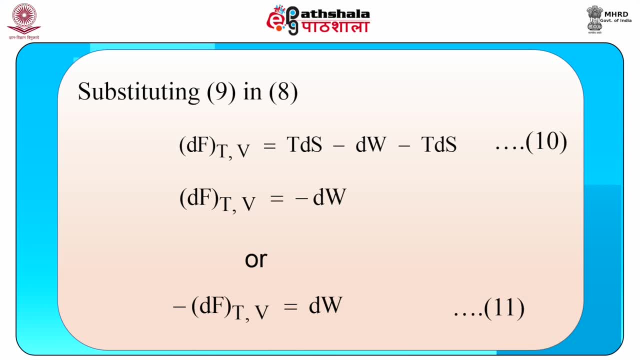 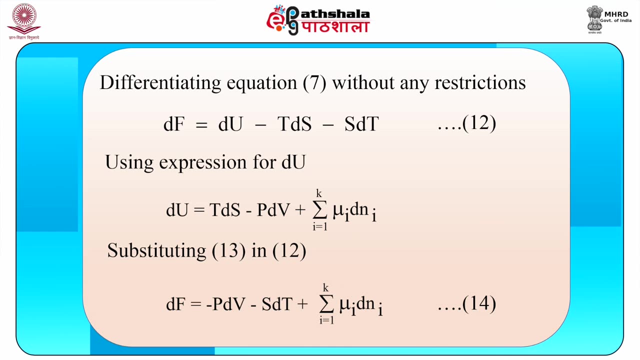 and volume. Therefore, total reversible work performed by the system is equal to decrease in Helmholtz energy at constant temperature and volume. Now differentiating equation 7, without any restrictions, we get dF as du minus Tds minus Sdt. Using expression for: 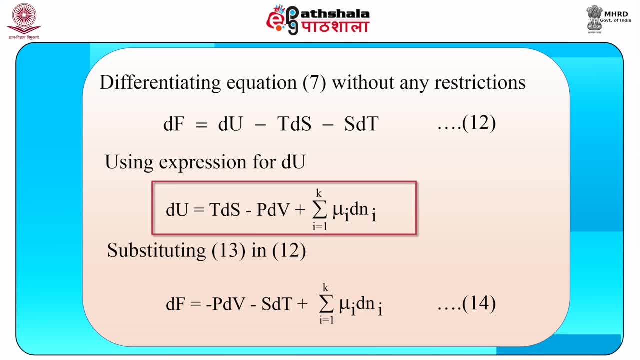 du as Tds minus Pdv plus. summation of mui dNi. we get the expression for dF as minus Pdv, minus Sdt, minus Tds, minus Sdt. So we get the expression for dF as minus Tds minus. 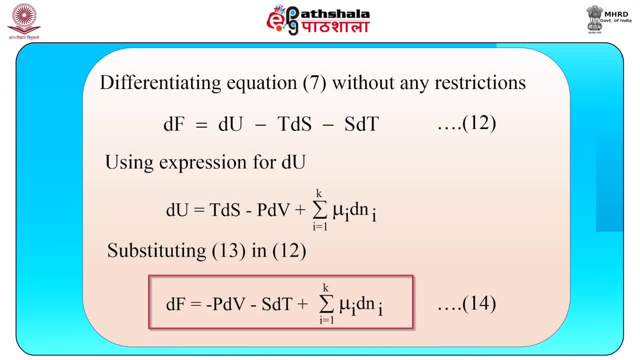 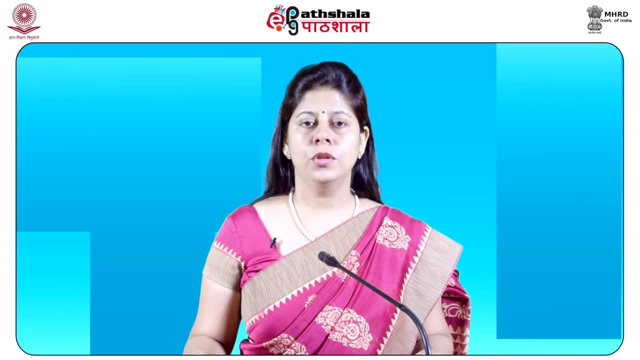 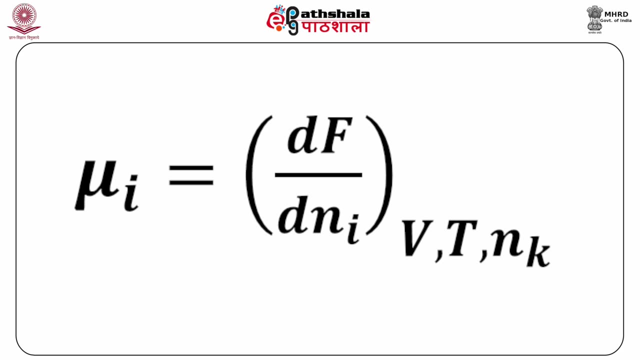 Pdv plus summation mui into dNi from i is equal to 1 to k. This equation gives new definition of chemical potential. Therefore we can write mui as dF by dNi at constant volume, temperature and number of moles of all other components, Gips, free energy. 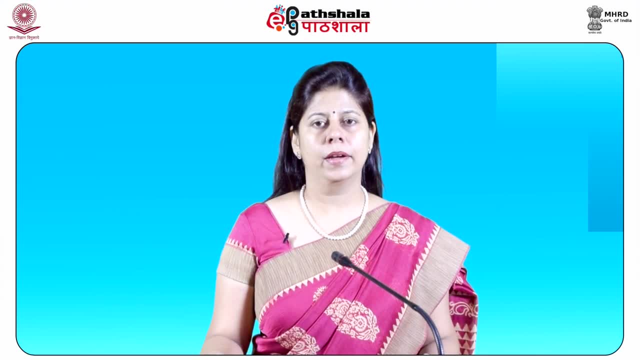 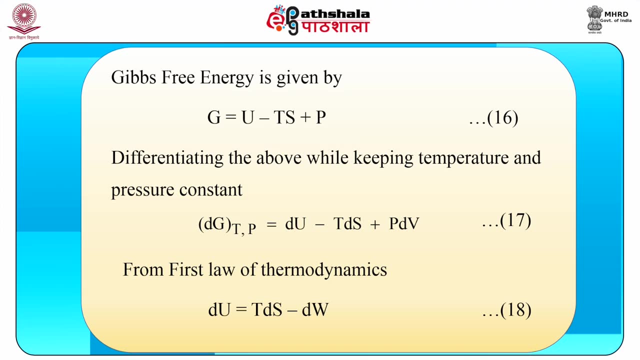 Where gips free energy is given by the expression g is equal to u minus Tds plus Pv. Diff the above equation. while keeping temperature and pressure constant, we get dG equals du minus Tds plus Pdv. From them. first law of thermodynamics, we have a relation: dU is equal toào. Therefore, 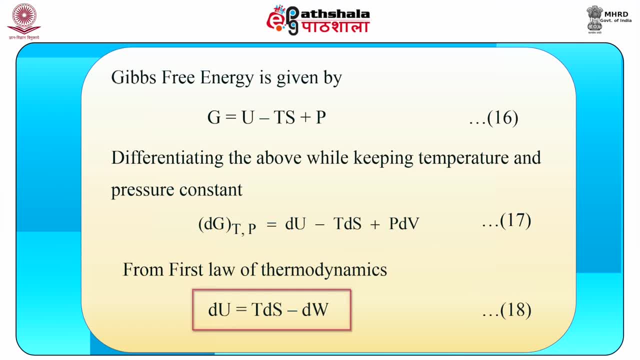 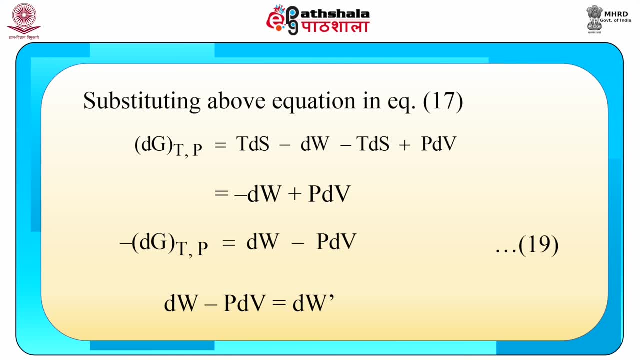 we have the equation for dF as du minus Tds minus Sdt. We keep present Relation twice and this ratio relates toget heavy From first law of thermodynamics. we have a equation Tds-Dw Substituting the above equation in equation 17,. we have Dg is equals to Tds-Dw-Tds. 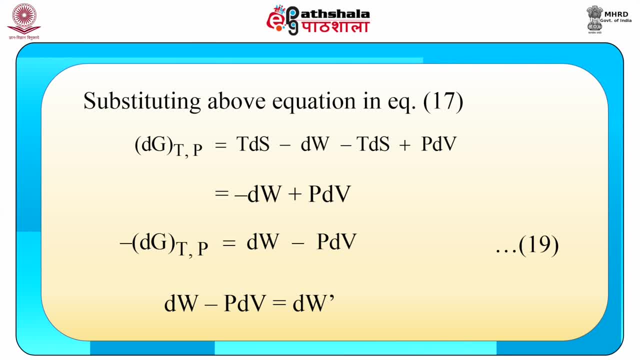 plus Pdv. Therefore we have the final expression: as Dg is equals to minus Dw plus Pdv, This equation shows the decrease in g is equals to total work minus the work of compression, which Gibbs call useful work, and Dw-Pdv is equals to Dw' It is that part of work which 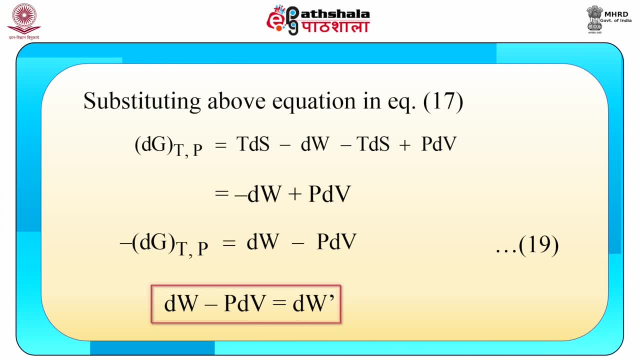 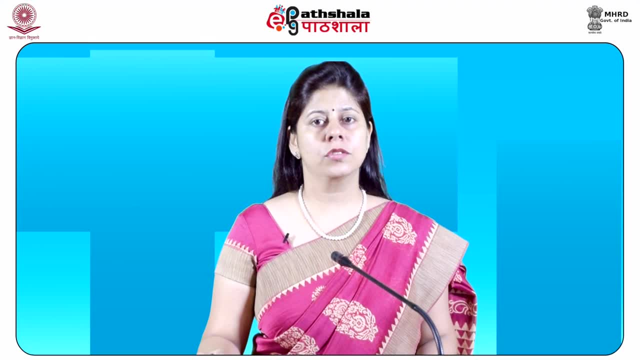 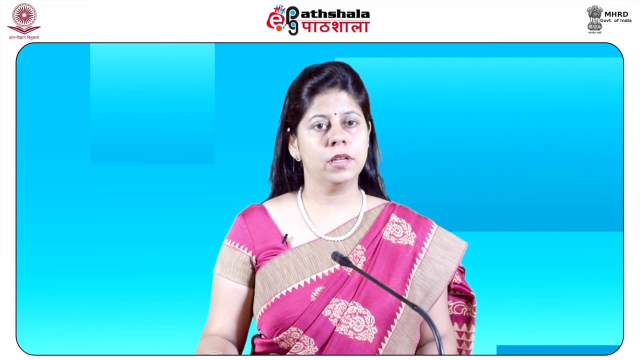 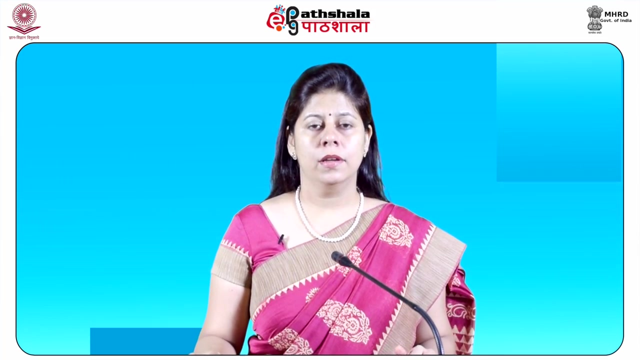 is contributed by chemical reactions or by the transport of electricity. In the study of condensation systems such as solutions, living tissues or solid material, PDV is usually small and generally does not contribute significantly to the total work, so that the choice of G 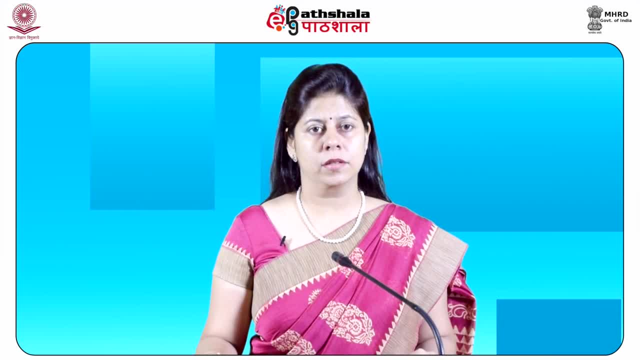 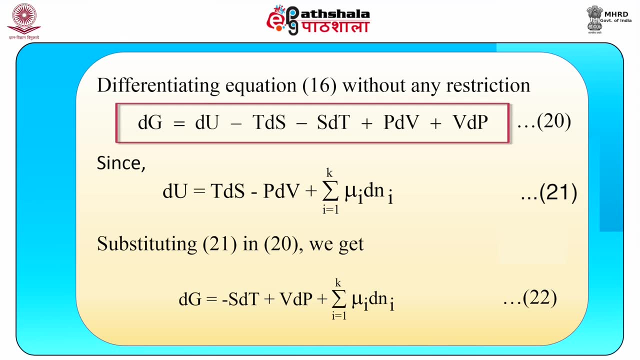 as the characteristic potential is common practice. Now, differentiating equation 16 without any restriction, gives dG as du-TdS-sdt-pdV-vdp, Since du is equals to TdS-pdV plus summation. mui dNi substituting this equation in equation. 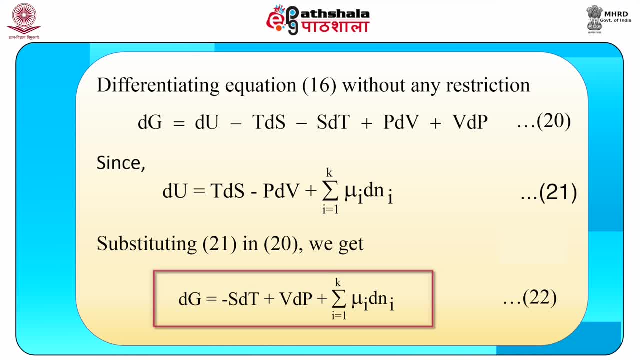 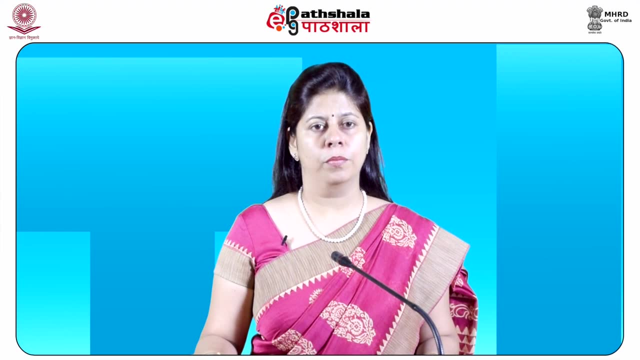 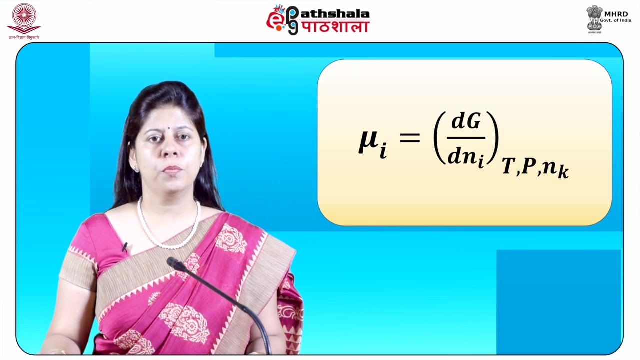 20, we get dG is equals to-sd2.. This expression defines the chemical potential in its most familiar form, ie. mui is equals to dG by dNi at the constant temperature, pressure and number of moles of all other. 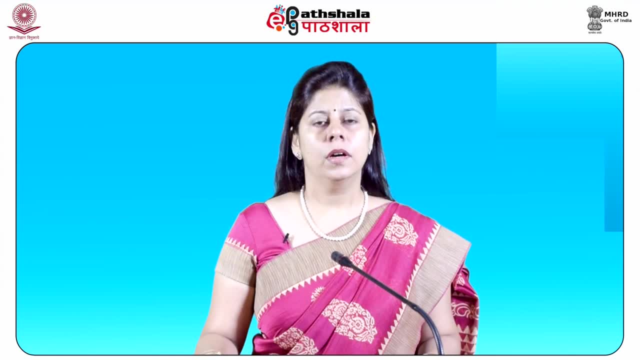 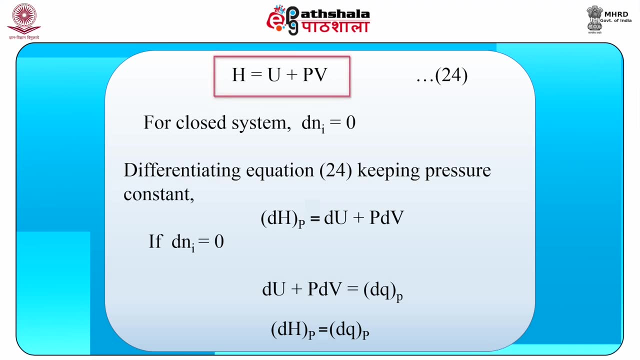 components: Enthalpy. Another common thermodynamic potential is enthalpy. It is defined as: H is equals to u plus pV. For the closed system, dNi is equals to 0.. Now differentiating this equation: keeping the pressure constant, we have, dH is equals. 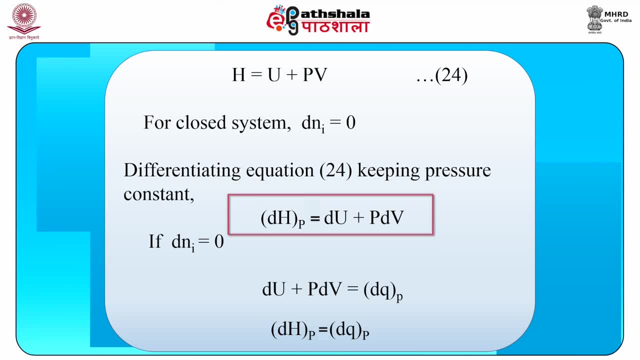 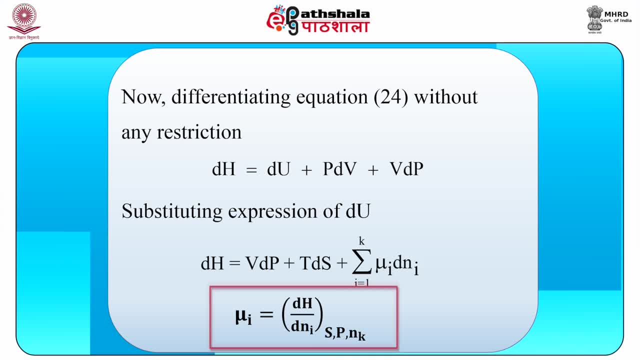 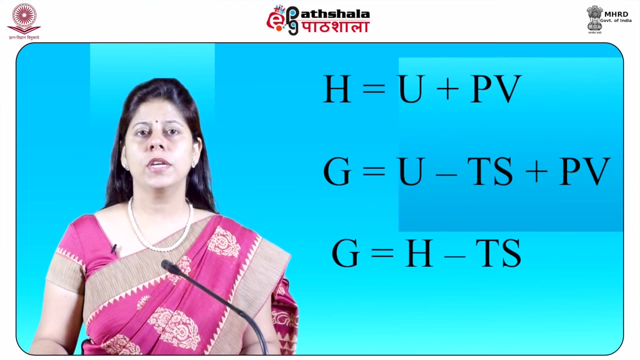 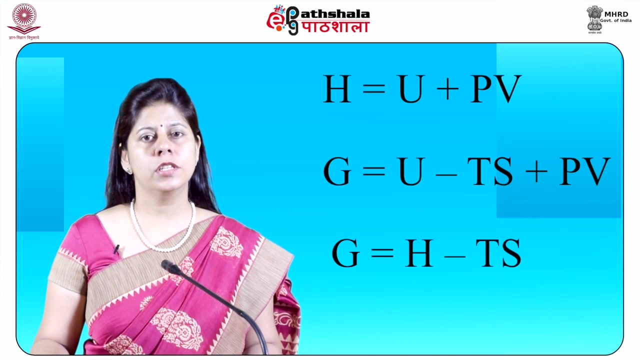 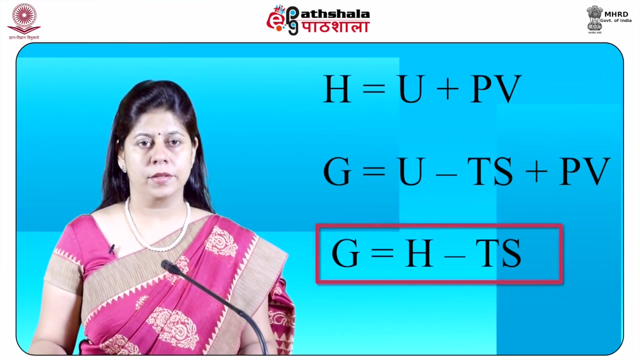 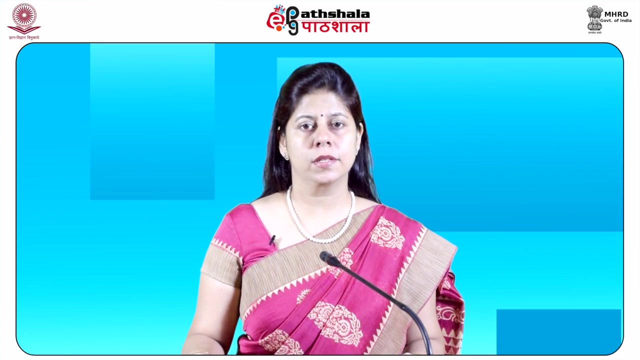 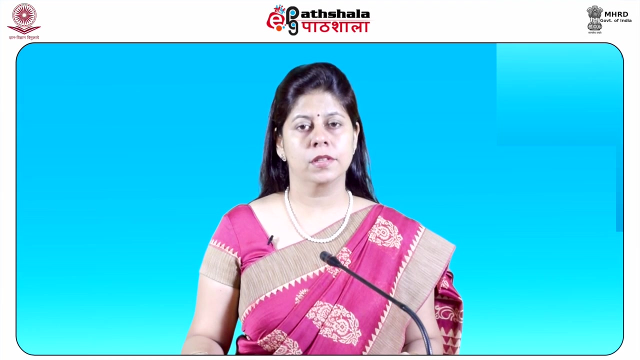 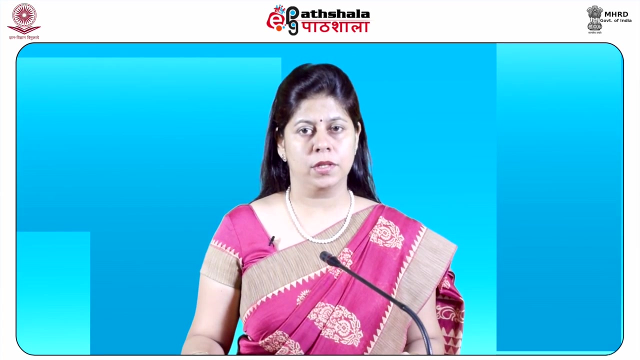 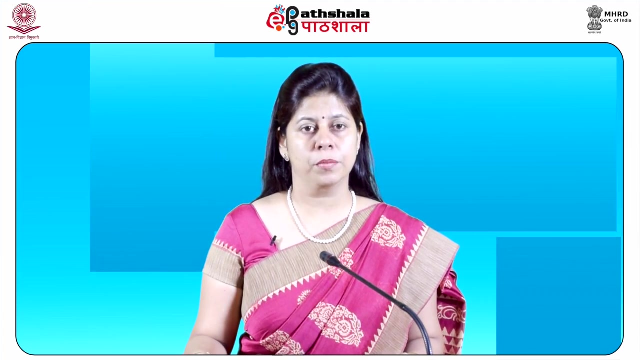 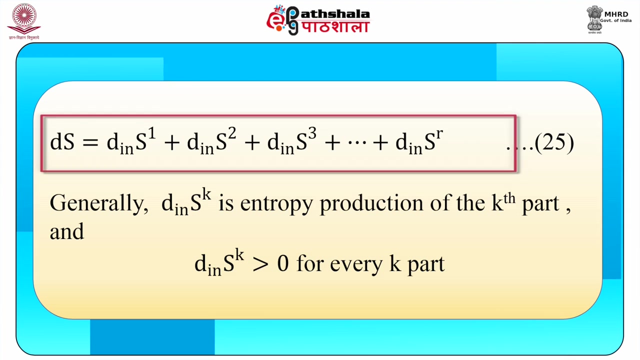 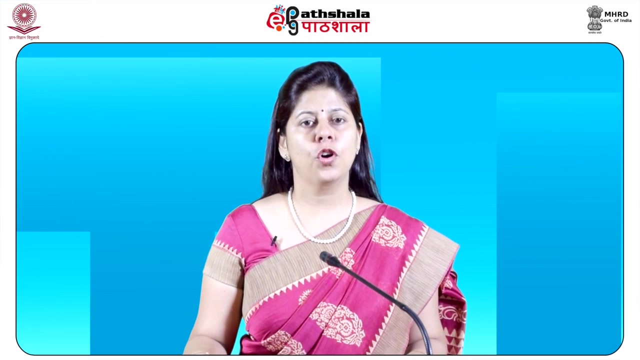 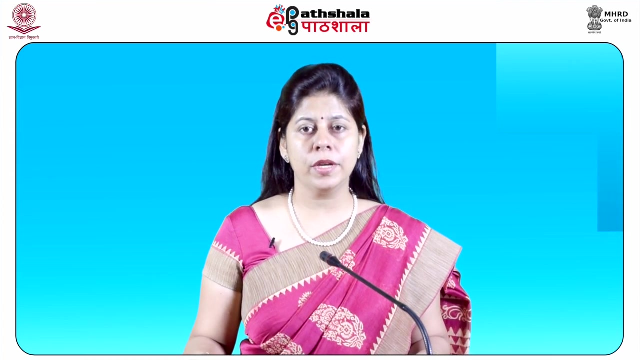 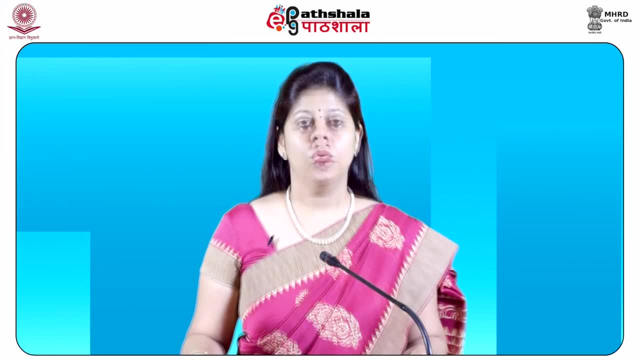 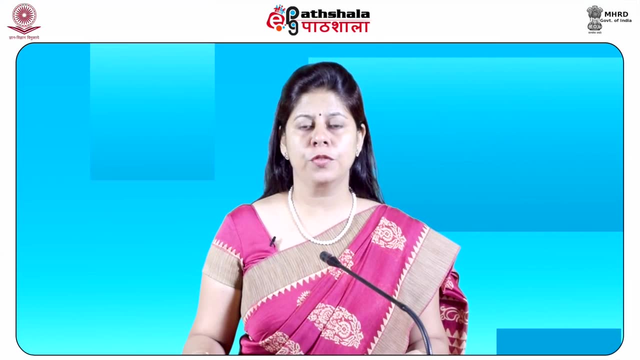 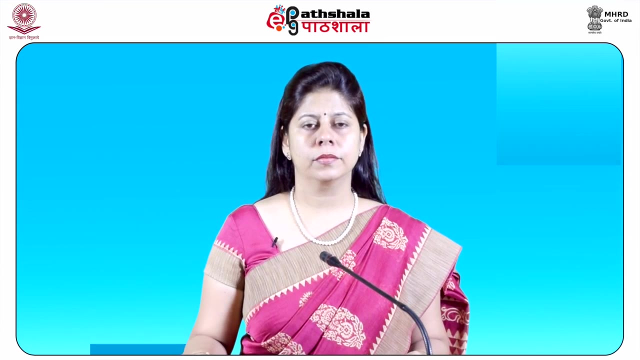 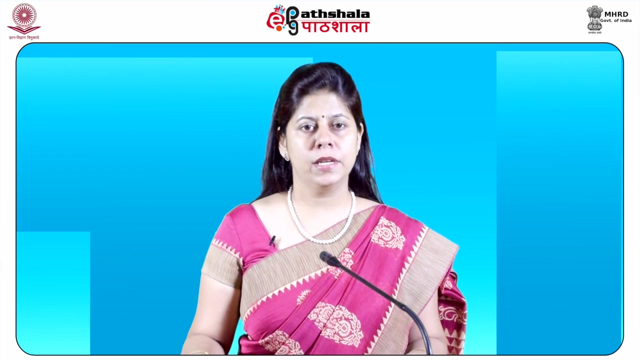 is equals to del q prime by t, where del q prime stands for the uncompensated heat, which is related as the production of entropy within the system because of some irreversible process occurring within the system. The thermodynamic potentials are: mu. i is equals to df by dni at constant vt and nk, which is the capital. The chemical potential in terms of Helmholtz free energy mu i is equals to dg by dni at constant pressure, temperature and nk, which is the chemical potential in terms of change in Gibbs. free energy mu i is equals to dh by dni at constant entropy, pressure and nk.